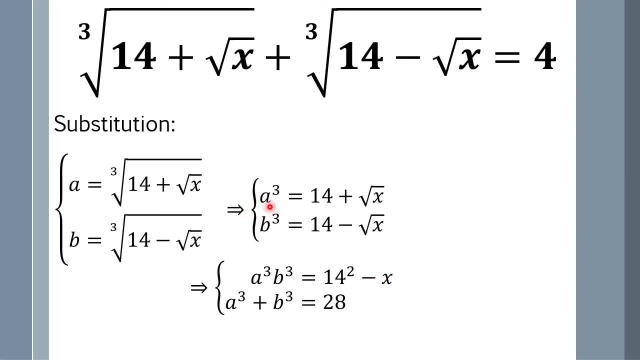 And if we add those two equations together, we have a cubed plus b cubed equals 28.. And on the x-axis we have a cubed plus b cubed equals 28.. And on the x-axis, we have a cubed plus b cubed equals 28.. 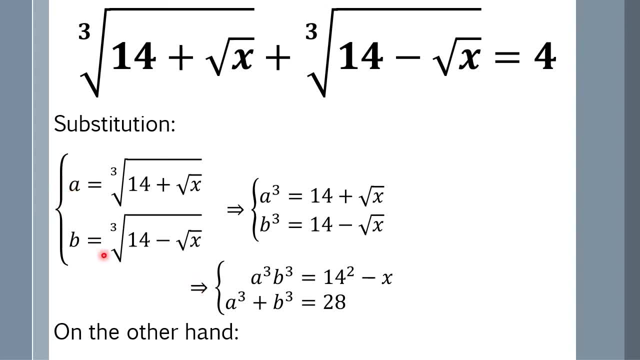 hand, by the definitions of A and B, we also have: A plus B equals 4.. So let's take another look of those three equations. From the first equation we can get X equals 196 minus AB cubed. Our job is to find the value of X. So if we are 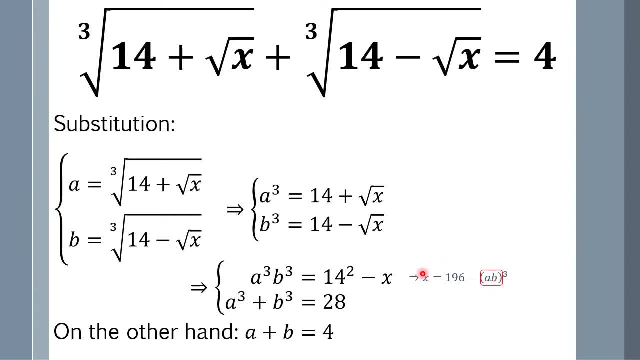 able to get the value of AB. we can find the answer of X. So our target is to find the value of AB based on the next two equations. Let's write down those two equations here: A cubed plus B. cubed equals 28.. A plus B. 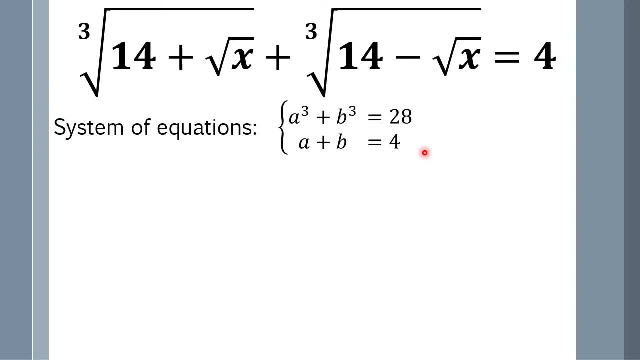 equals 4.. There are different ways to solve these system modifications, but here I would like to introduce the concept of symmetric polynomials. A symmetric polynomial means: in this polynomial, if you switch any two variables, the expression remains the same, Apparently. 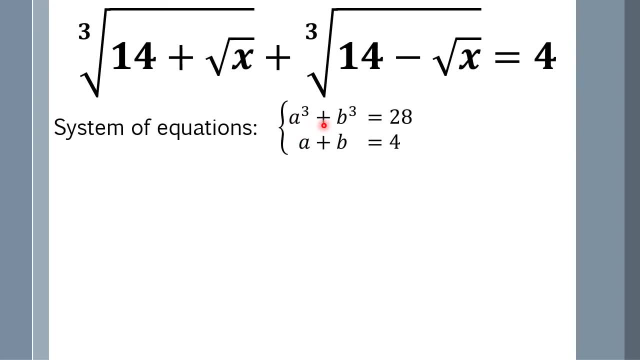 in this question. A cubed plus B cubed and A plus B are both symmetric polynomials. In algebra there is a very important theorem. It states: any symmetric polynomial can be written as a polynomial expression of elementary symmetric polynomials For a two-variable.